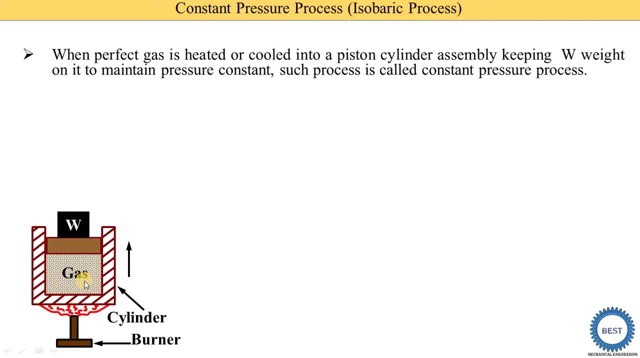 by using the burner, the gas state is changed And due to that their piston is changed. so we need to try to move in upper directions For this, maintaining this constant pressure. here we putting this W weight. Now we draw the PV diagram On the x axis. that is a volume. is there? 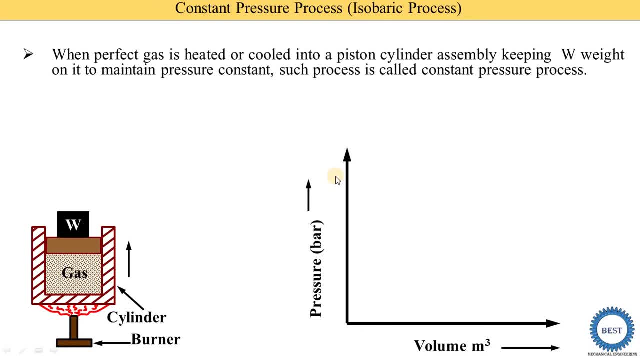 and unit of the volume is meter cube. On the y axis pressure is there and unit of the pressure is bar. So first we putting this state number 1.. State number 1 means the pressure and volume of the gas at the initial condition, means when we are not supplying this heat energy. So we get this point. 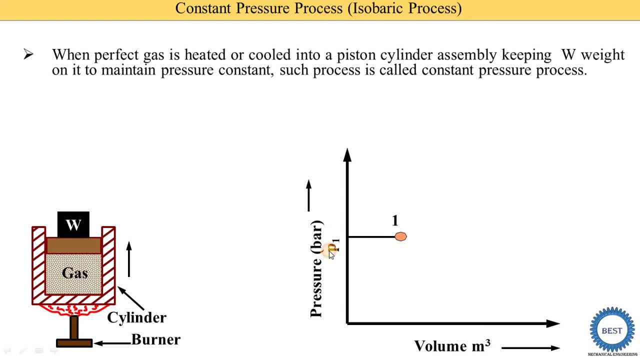 and at this point it have the certain pressure. So pressure is P1, it have certain volume, it is called as the V1.. And then, after we start to supply this heat energy by the burner, at that times the state of the gas is changed. And when this state is changed, at that time 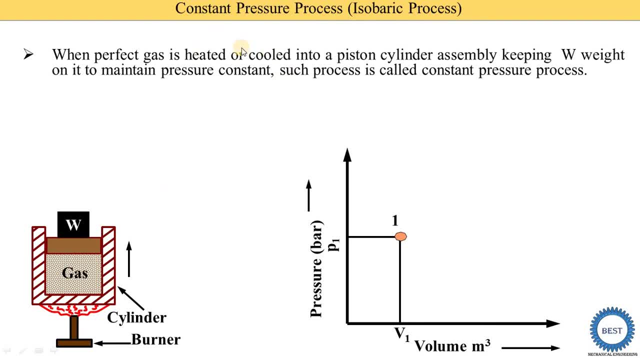 the pressure is remains constant. Here we see that is a constant pressure process. is there That means the pressure is remains constant. When we draw this horizontal line from the point 1, at that time the pressure is remains constant, Because this pressure is on the y axis. So in which side? 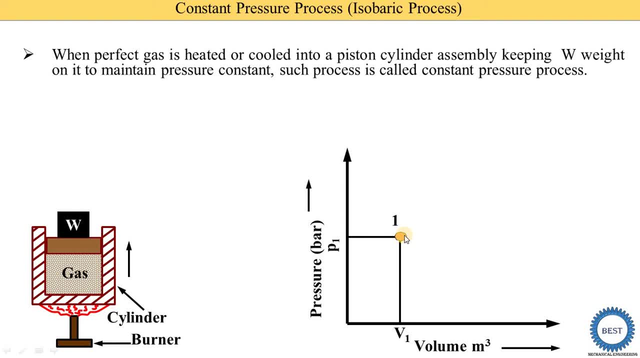 we draw the horizontal lines, We have the 2 option: either we draw the horizontal line from the point 1 in a left directions or the right directions. It is depend on the heating or cooling process. So here we are, doing this heating. When we do the heating of the gas, its volume is increase. 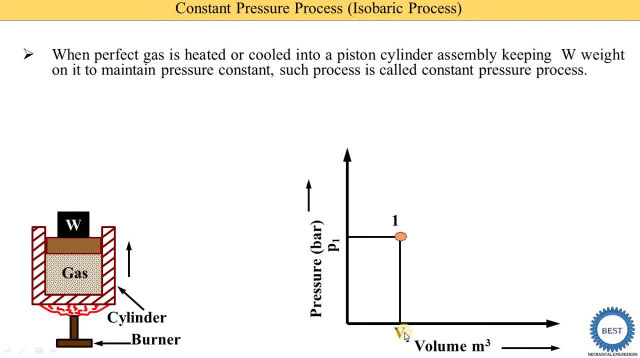 x-axis. when we moving on the right side, the volume is increased. okay, so our line is moving from left to right sides and it is the point number two, and at the point number two pressure is equal to p2. so this p2 is equal to p1 and hits have certain volume. that is called the. 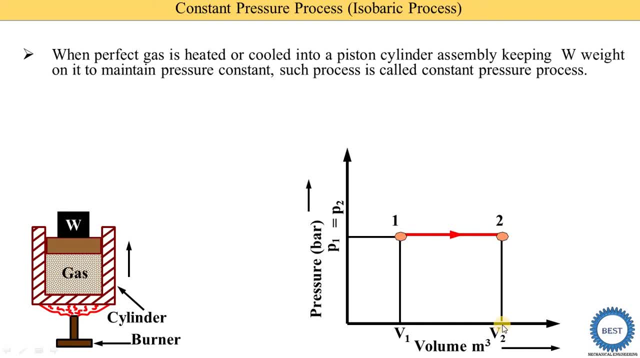 volume v2. okay, so this is the basic things about the constant pressure process, and area under the pv diagram is denoted as the amount of work done by the system or required by the systems. okay, so it is depend on the heating or a cooling process. so when we do the heating, 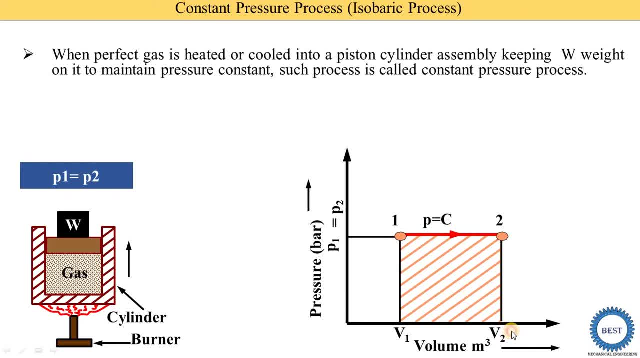 of the system at that time, system is produce the work done okay. and when we do the cooling of the system, at that time we require to supply the some work done okay. so here we are doing this. heating means system is produce some work done because this weight is lift the. 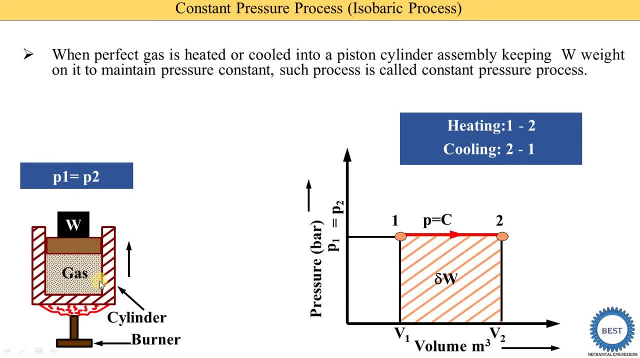 weight is moved In this upper direction means some work is produced by this gas. okay, so it is considered as the positive work. when the cooling is there, at that time, the work is required by the system. okay, so when this cooling process is carried out, at that time this process is flow from. 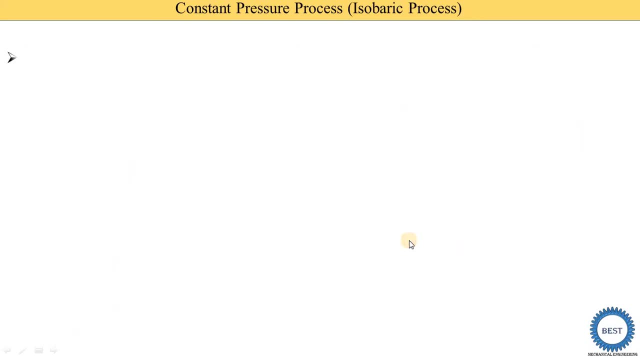 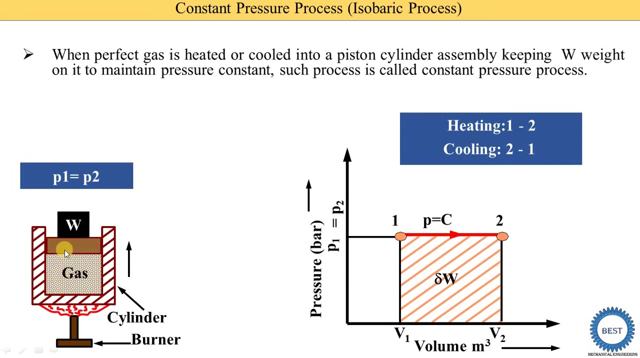 the state two to state one means this arrow is change the process will result in an increase or decrease in the volume. okay, so here we already studied. The volume is increase or reduce means. suppose the heating is going on, then the volume is increase because when we heat the gas its molecules are move with the higher speed. okay, 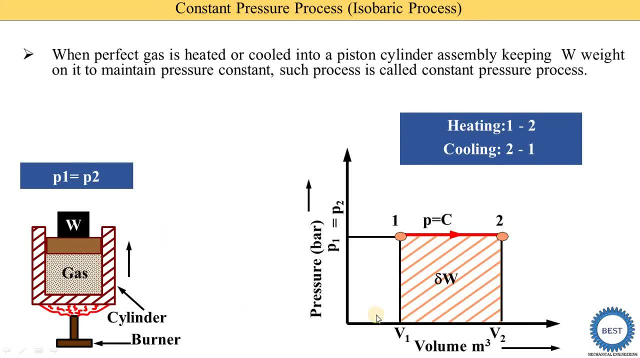 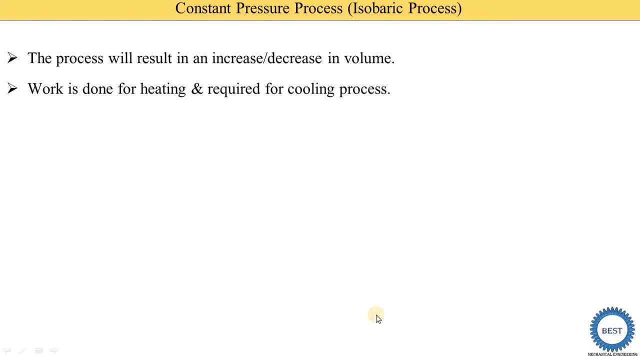 that's why its volume is increase and when we do the cooling, the volume is reduce. work is done for heating means when the we supply this heat energy system give some output- okay, and when we do the cooling, at that time we need to supply some work done to the systems. 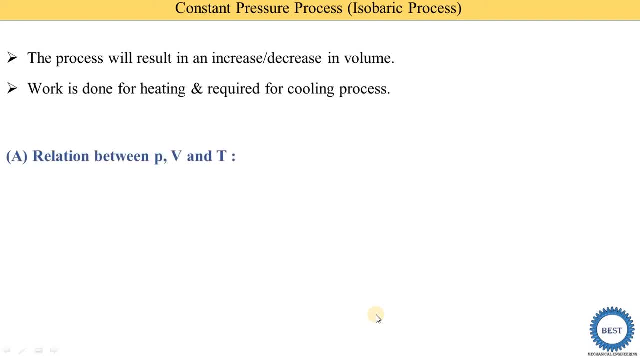 now we find out this relationship between the pressures- Okay- Volume and temperatures. so basic equation is that the p one v one divided by t one is equal to p two, v two divided by t two. but here we know that we are studying the constant pressure process. that means the p one is equal to p two. okay, so we cancel this p one, p two. 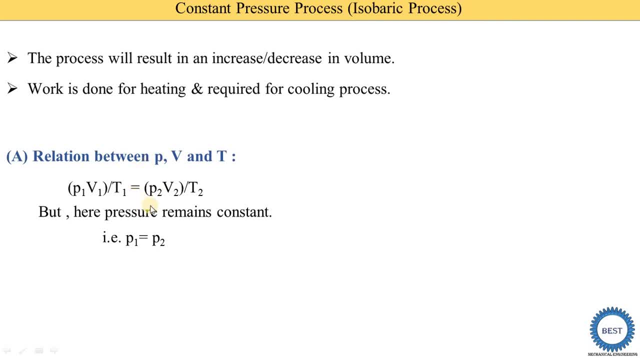 because its value are same. means how we cancel we putting this by: replace the p two by p one means both the side. p one is there, so we cancel it, okay. so what is remaining parts? remaining part: So we have the v one divided by t one is equal to v two divided by t two. so this is: 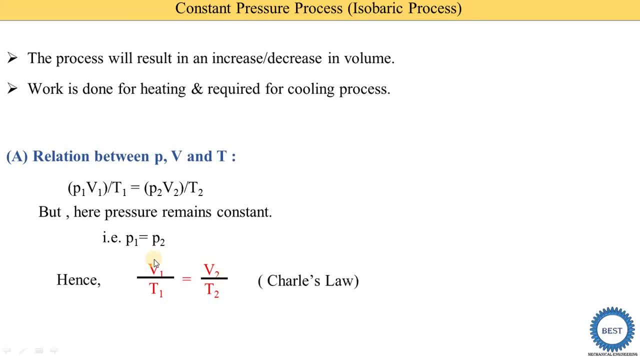 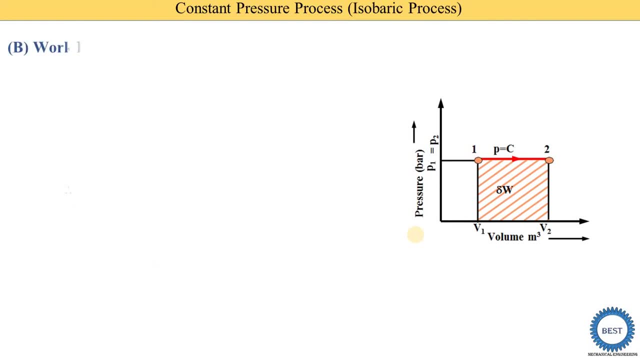 the relationship between pressures, volume and temperature, and it is also called as the charlestow means the constant pressure process is followed a charlestow now. second, we derived the equation of work done. so when we study about the constant volume process, we know that the work done produced during the constant volume process is zero, because in a p-v diagram, 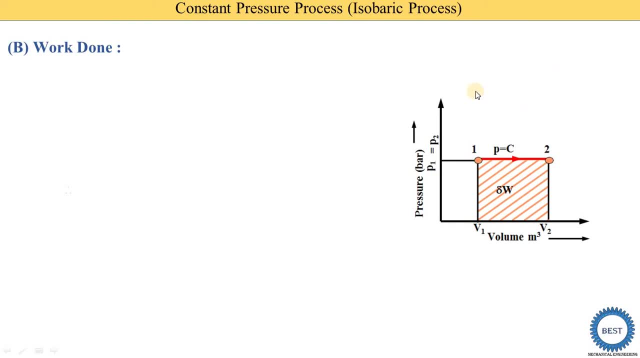 area under the line is zero during the constant volume process. okay, so in a constant volume process we draw the vertical line. okay, so in a vertical line there is a zero or zero area is there. that means the work done is equal to zero, but in a constant. 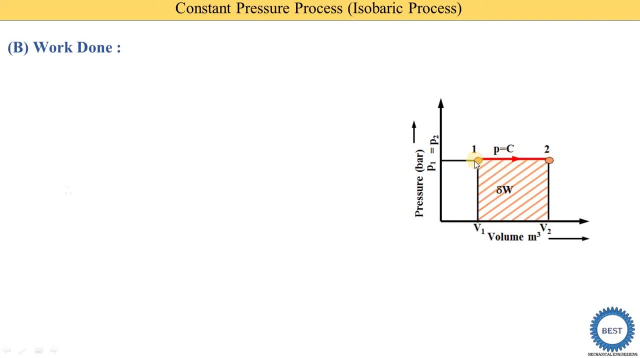 pressure process. here you see it is. it's have a certain area under these lines. okay, this one to two line is indicate the constant pressure process and this is some area is there and what is this area of this rectangle for a square? okay, so how we find out this area of the square? so first we need 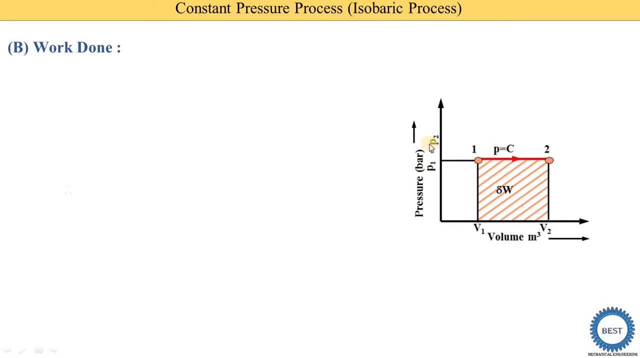 to measure the height. what is the height height? is the p1 or a p2? both are same, okay, so we consider it is the p. how we find out this width? so find out this v, we need to. we need to do the subtractions of this two volume, that is, the v2 minus v1. then we know this weight. okay, so work done is equal. 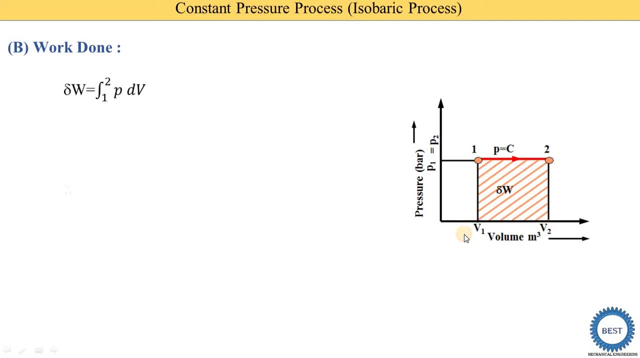 to pressure in bracket v2 minus v1. okay, so this is the simple way to write down this equation of the work done from this pv diagram. okay, we can also find out by this way that is, the work done is equal to integration into pdv. okay, so integration of the pressure is. 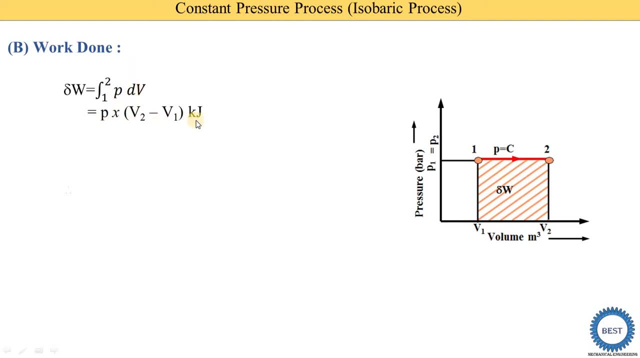 as it is and the integration of the dv is v2 minus v1 and unit is the kilojoule, okay. so i written again the same equation. that is the area under the curve, so area under the curve is the square, so we measure the height. height is the pressure, okay, and the width is the v2 minus v1. 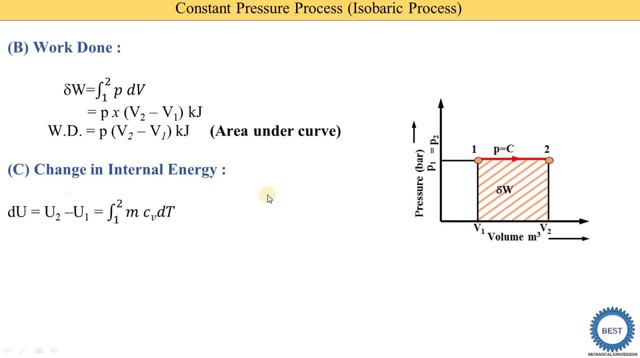 next we find out the change in internal energy. so change in internal energy is denoted as the du. okay, so change in internal energy means we need to do the subtractions of the two energy: one at the internal energy at the final state, minus internal energy at the initial state. 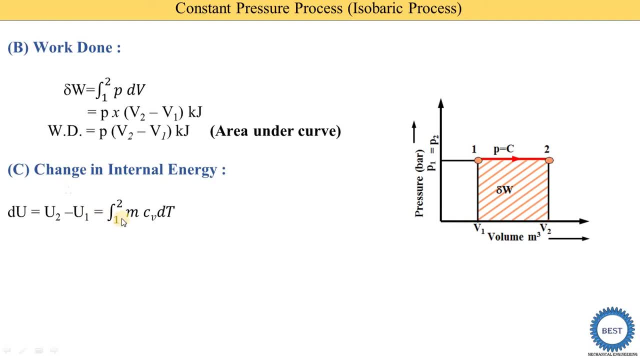 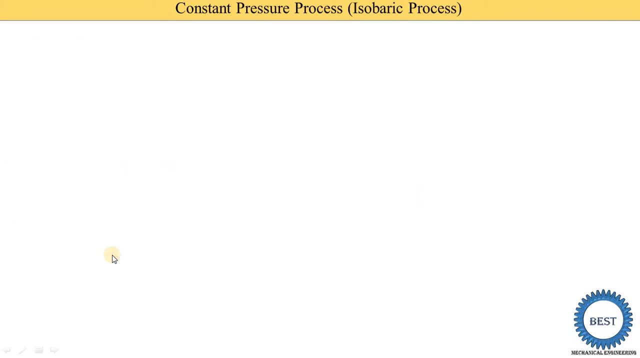 okay, so it is the u2 minus u1 is equal to integration mcv dt. okay, so when we do these integrations of the dt we get it is the t2 minus t1 means the final state temperature minus initial state temperatures. okay, so this is the equations of the change in internal energy. that is the. 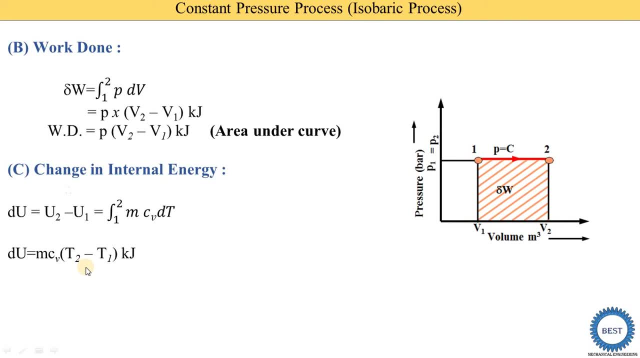 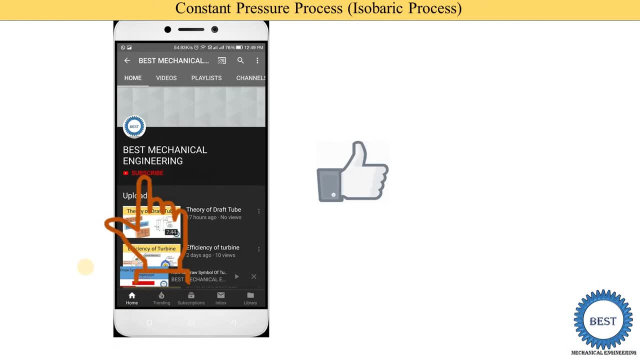 internal energy is directly proportional to the change in the temperatures. now, before moving ahead, i request to like the video and subscribe my channels for watching the more video related to bme or eme. subject or engineering thermodynamics for bme or eme. various link is provided in. 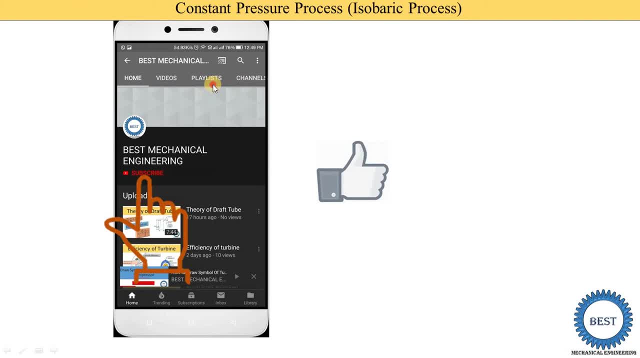 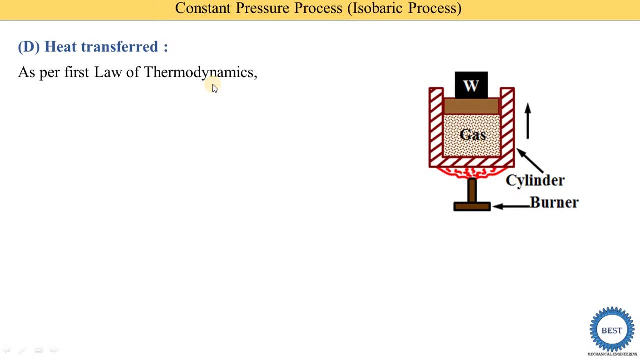 descriptions, as well as in the car for other subject. i request to visit the playlist now. next we find out these equations of the heat transfers. okay, so as per the first law of the thermodynamics, the heat energy is equal to work done, plus change in energy means. here we supplying. 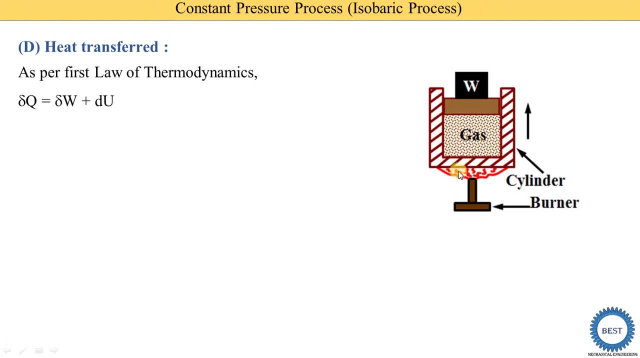 this heat energy. okay. and this heat energy have the two options: okay. either it is converted into some work dance or either it is stored in this form of the internal energy. that's why the q is equal to work plus internal energy. okay, so we know the equations of the work done and the change in. 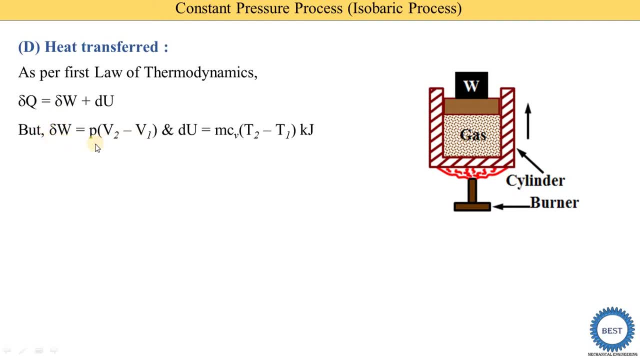 internal energy in the editorial bme: okay, so dot t is already performed. okay, so there is a p which is equal to work and that we find already find out. okay, so we find out. this work done is equal to p. in bracket v2-v1 we also find out change in internal energy. that is mcvtwo t minus t one, so we're. 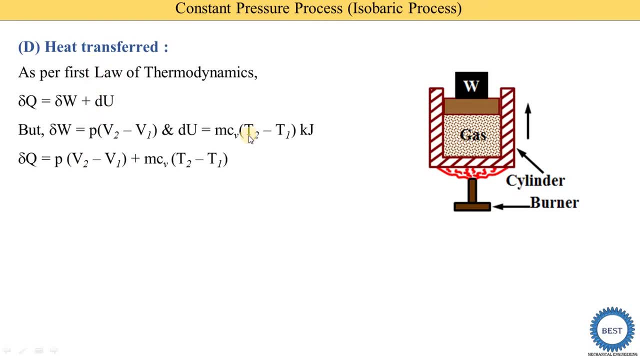 putting this value in these above equations: okay, so we're putting this value of the work, that is, the p, in bracket b2-v1, plus we putting this value of change in internal energy: mcv two minus t one's. okay, then we're putting this value of this term, so we know that the pv is equal to. 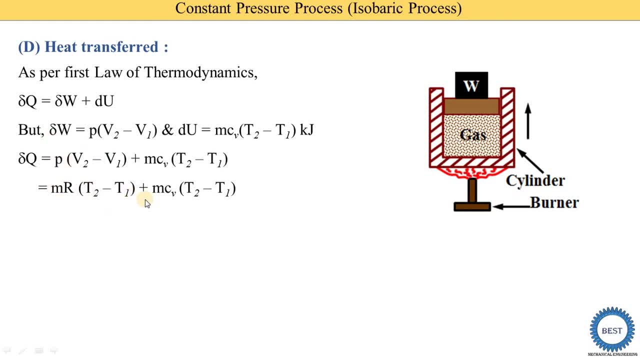 mrt. okay, so by using mrt. okay, so by using, is relationship. here we putting that mr is equal to t2 minus t1 plus the under the term is: as it is. okay, then we know that this r is equal to cp minus cv. okay, so we replace this r by the cp minus cv. 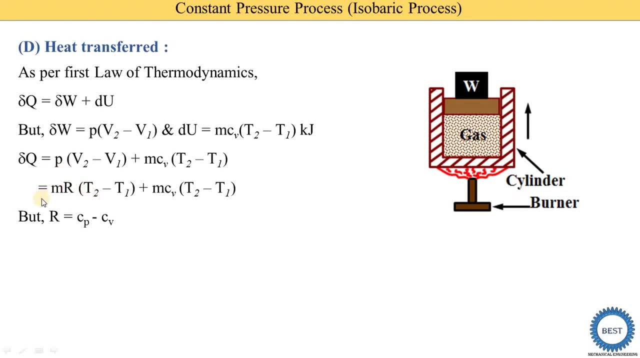 okay. so when we replace this r by the cp minus cv, then we get the two term. one term is the m cp in bracket, t2 minus t1. we get second terms, that is a minus mcv, t2 minus t1. okay, so here plus mcv, t2 minus t1 is there. so they are cancels, okay. so what is the equations of the? 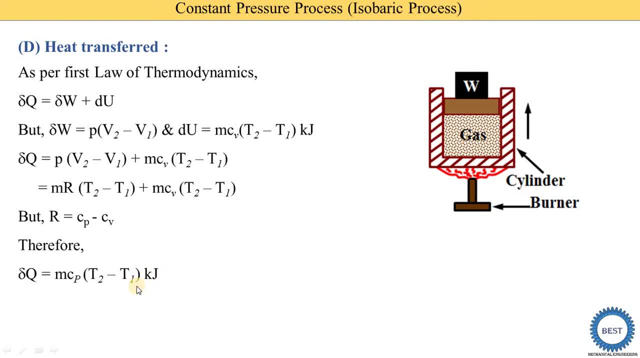 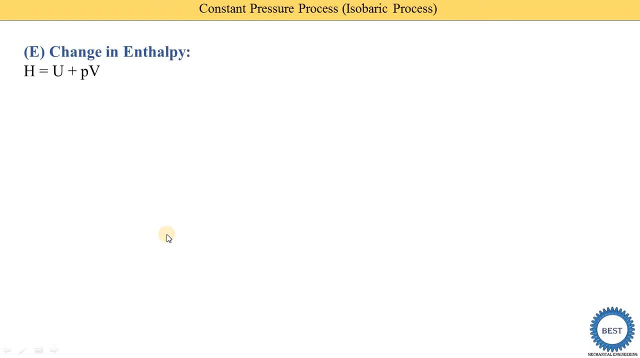 heat transfer. that is the mcp t2 minus t1 in the kilojoules. okay, now, next we find out this change in the enthalpy. so change in the enthalpy means that is the enthalpy at the final state minus enthalpy of the initial state. okay, so what is the equations of the enthalpy? enthalpy is equal to: 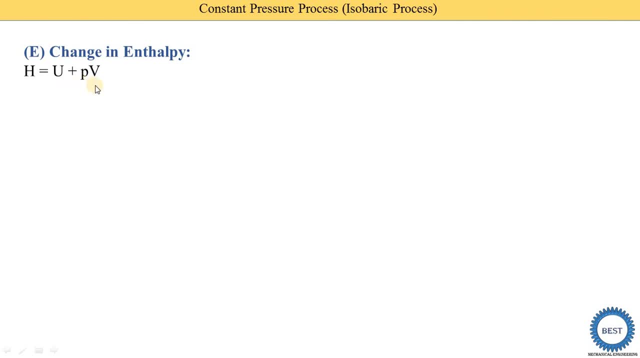 internal energy plus flow work. internal energy is u, flow work is the pv. okay, so we write down this equation of the enthalpy for the initial state and for the final state. initial state of the enthalpy is the u1 plus p1- v1. final state is the h2 is equal to u2 plus p2 v2. okay, so 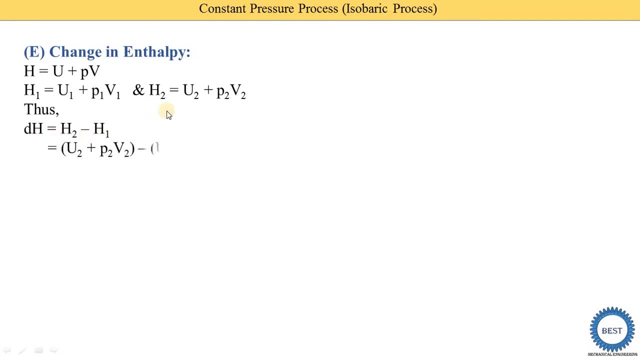 change in the enthalpy is the h2 minus h1, so we have the value of h2. that putting here that is u2 plus p2 v2 minus h1, that is the u1 plus p1 v1. now we do the some modification in this equation. 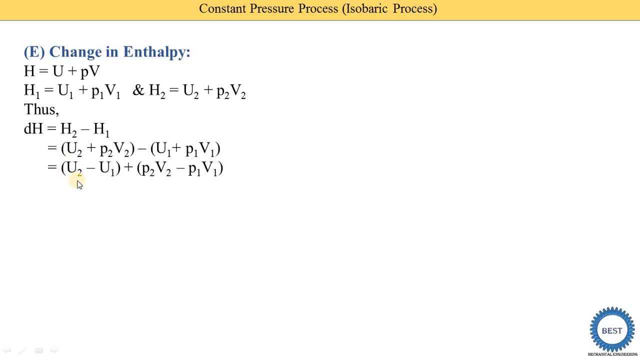 that is, we are gathered the same parameters means internal energy. that is u2 minus u1 plus. in another bracket we mentioned this flow work that is a p2 v2 minus p1 v1. okay, now this u2 minus u1 means that is a change in the internal energy. okay, so we also know that is equation of the change in. 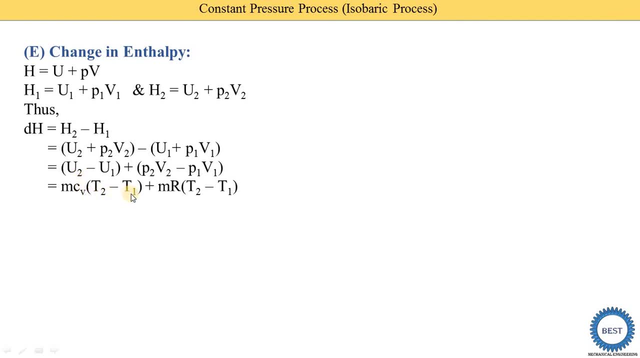 internal energy that we derived earlier, that is the mcv. t2 minus t1. okay, means this: u2 minus u1 is du, okay, so here we putting this value of du, and we also know that the pv is equal to mrt. okay, so p2- v2 is equal to mrt2. p1- v1 is equal to mrt1. so we get this, mr in. 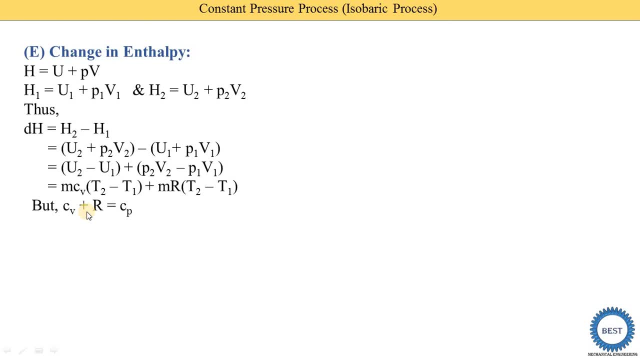 bracket t2 minus t1. okay, now we change some parameters here. that is, we know that the cp is equal to cv plus r. okay, or r is equal to cp minus cv. that we do for the change in internal energy. so here we replace this r by the cp minus cv. okay, so this cv cv step is cancels and we get this. 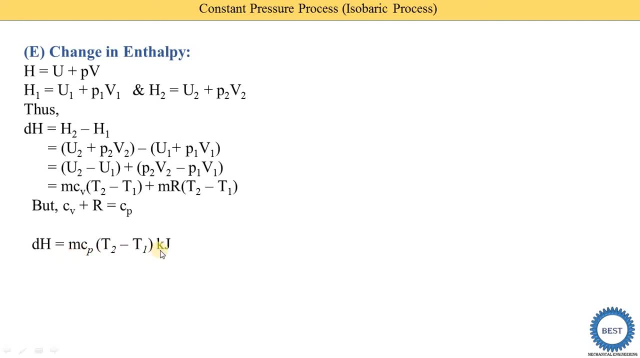 change in the enthalpy is equal to mcp t2 minus t1 in kilojoules. okay, so means here we replace this r by the cp minus cv. okay, so we get two term from this equation, that is the m? cp in bracket, t2 minus t1. other step: we get the minus mcv, t2 minus t1. so here plus mcv.